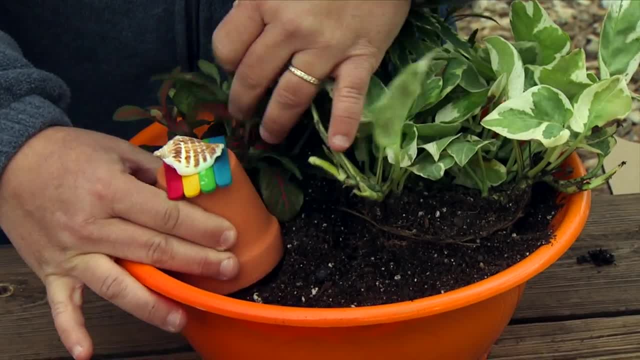 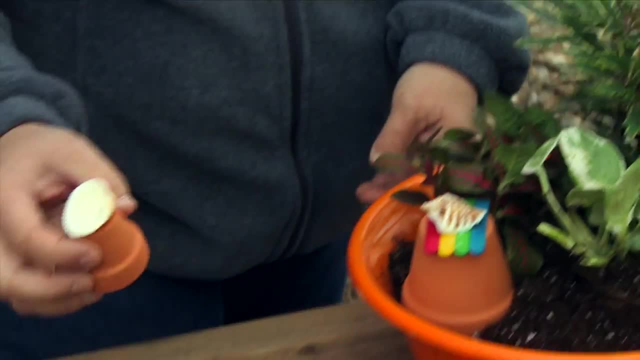 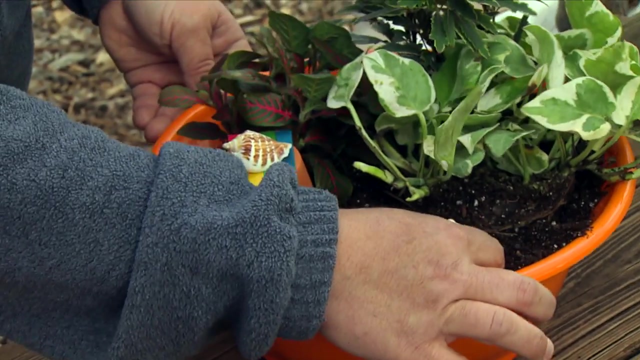 fun. I'm going to nestle it over here on the side. and then I made a bird bath which it even holds water, and some kids in the past have actually painted it blue or put little blue beads in it. So I'll put that over here and then you can make a garden path. You can get some. 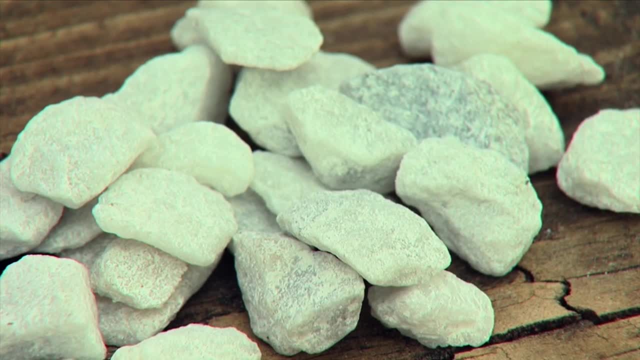 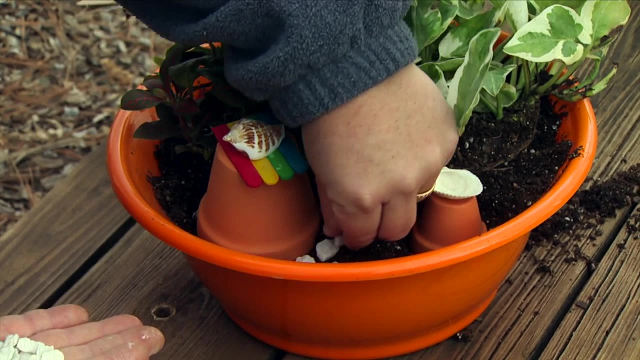 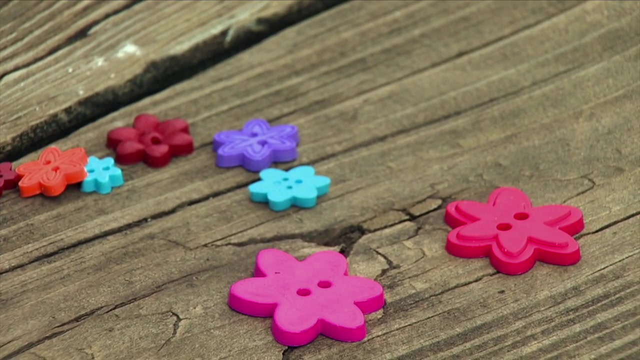 aquarium gravel or some marble chips and you can just make a little sidewalk path. If you want, you can add some flowers to your little gnome garden. So I just got some flower shaped beads and fun little colors And I'm just going to spread them around- Instant flower garden. 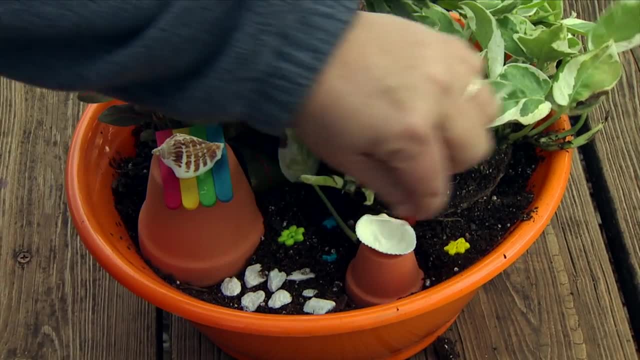 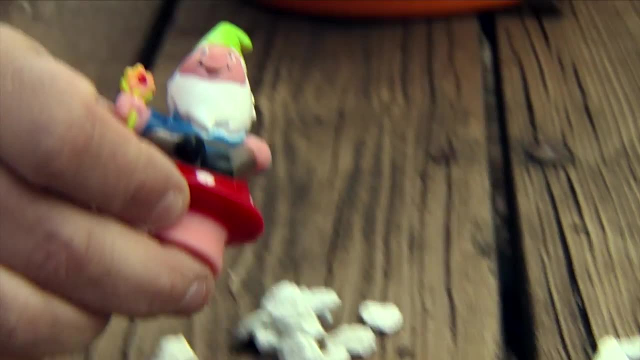 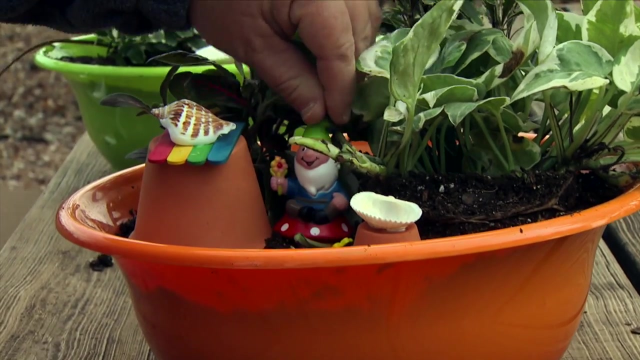 Put some behind the flower just for a little fun bits of color. And then the owner of the little gnome home is Mr Gnome, Mr Jerome the gnome, and he's going to just sit right next to his house, or you could use all those McDonald's toys that are piling up in the 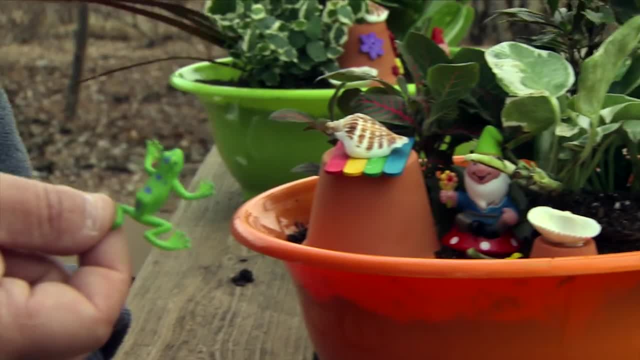 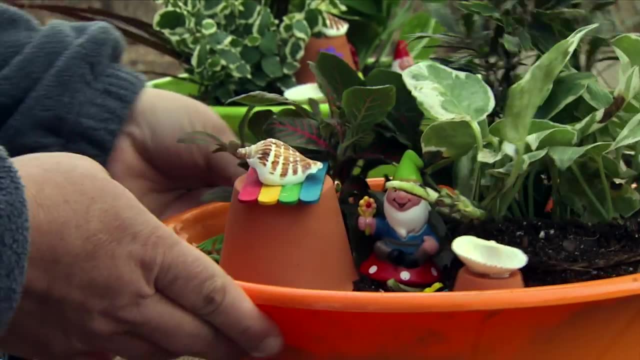 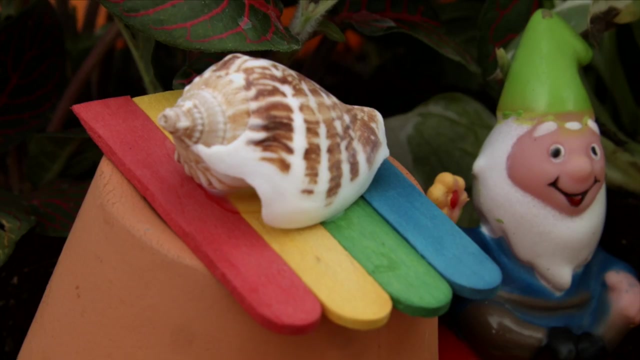 bottom of your kids toy chest. And then, just for fun, I also have a little plastic frog. There's plastic insects, whatever you want, and you can just hide him back in here. So this particular garden didn't have much room left, but depending on which size plants you use, 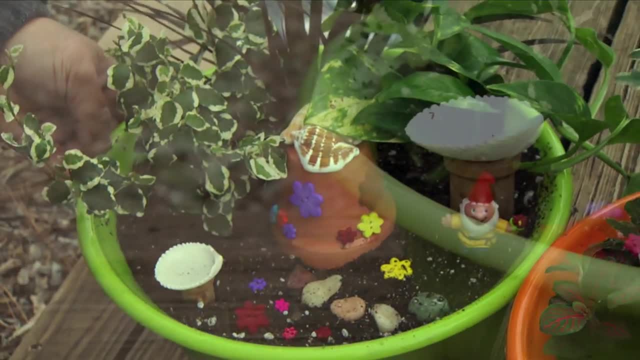 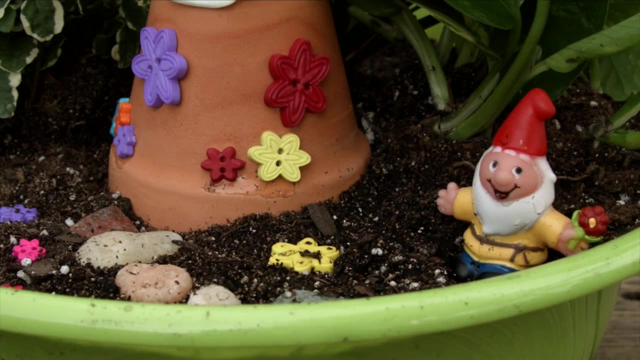 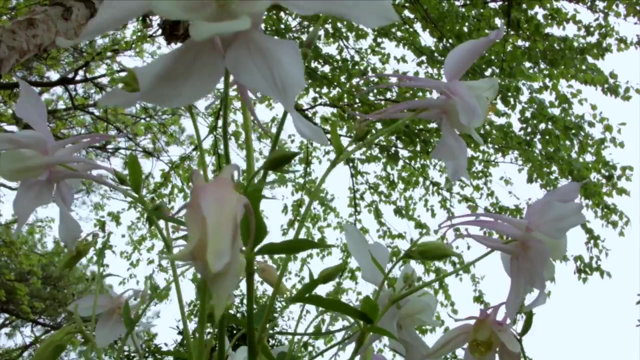 you can have more room to mess with, or you can put in fewer plants or smaller plants, But eventually they're going to grow and you're either going to need to transplant them or take out the gnome. But it's a fun little project you can do with kids. 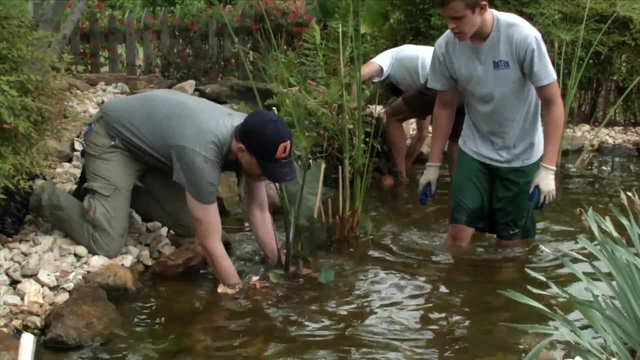 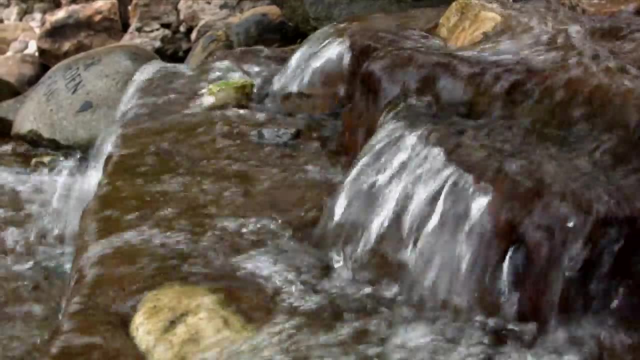 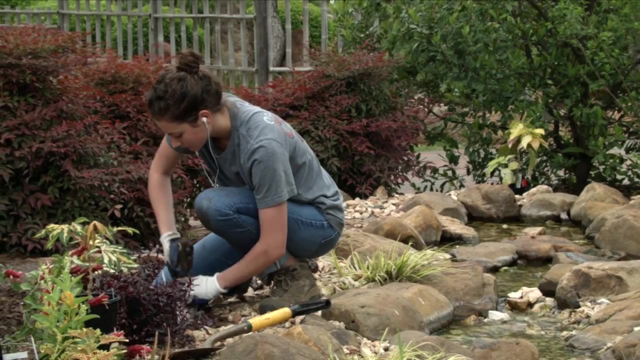 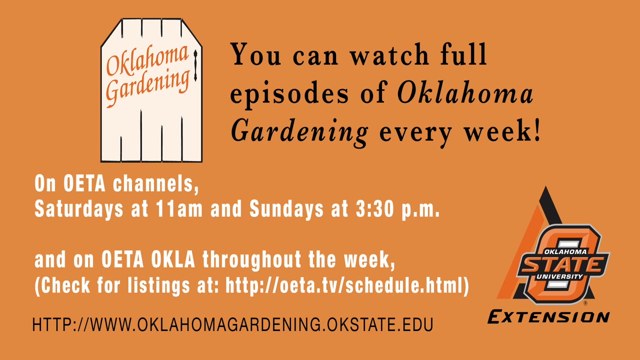